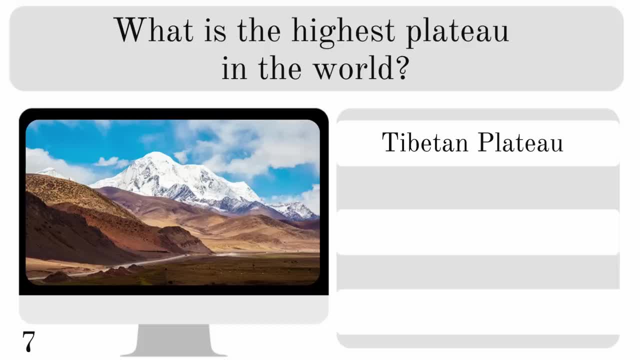 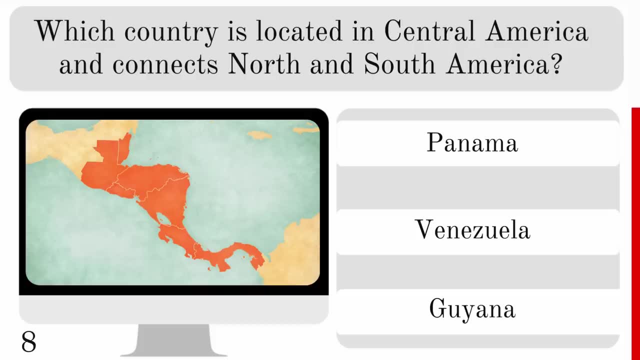 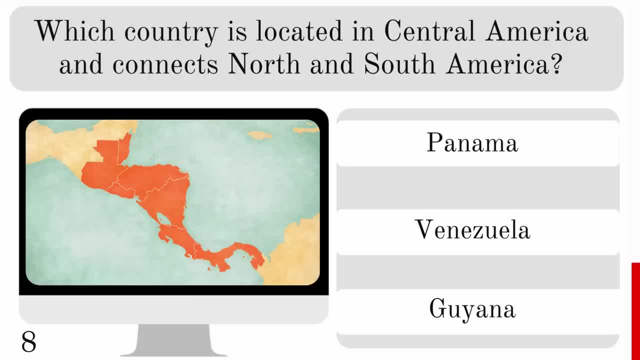 Which country is located in Central America and connects North and South America? Is it Panama, Venezuela or Guyana? Which country is located in Central America and connects North and South America? Is it Panama, Venezuela or Guyana? The correct answer here is Panama. 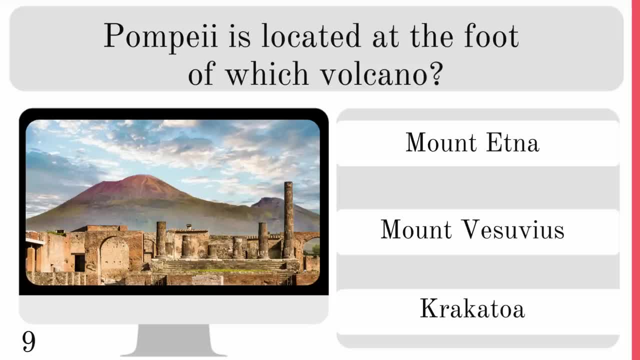 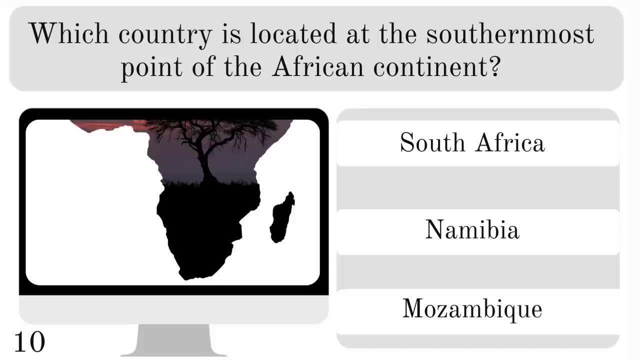 Pompeii is located at the foot of which volcano? Mount Etna, Vesuvius or Krakatoa? And the answer is Mount Vesuvius. Which country is located at the southernmost point of the African continent? South Africa, Namibia or Mozambique? 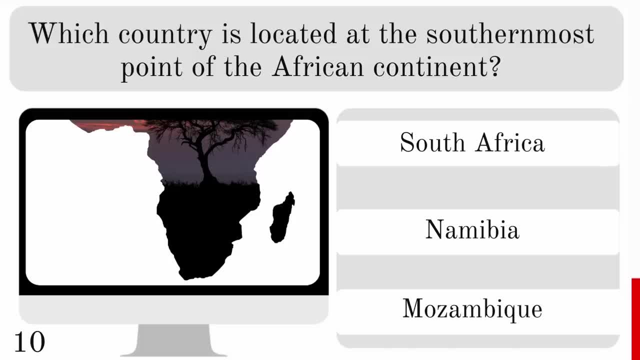 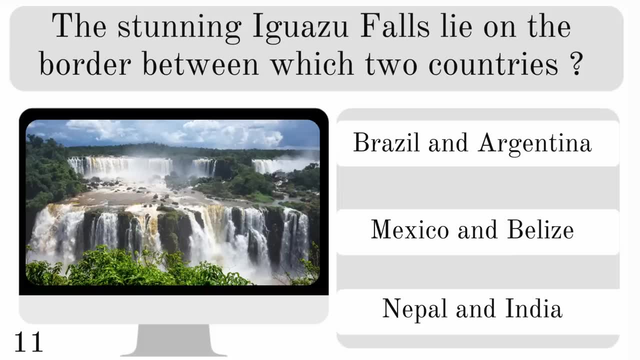 Mars or Mars? WOW, that's quite a huge list And the correct answer there, South Africa. The stunning Iwazu Falls lie on the border between which two countries, Brazil and Argentina, Mexico and Belize. on Nepal and India. Yamunada falls under Bermuda, curcuma or Burly Manom. 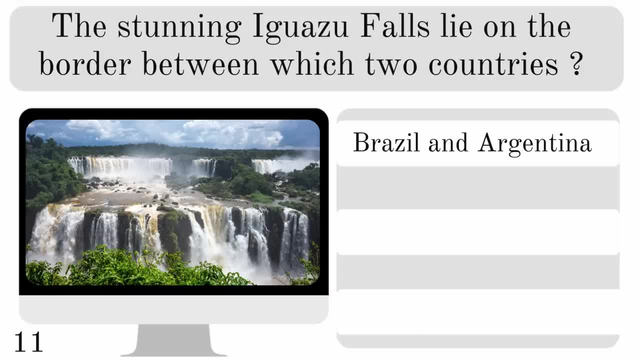 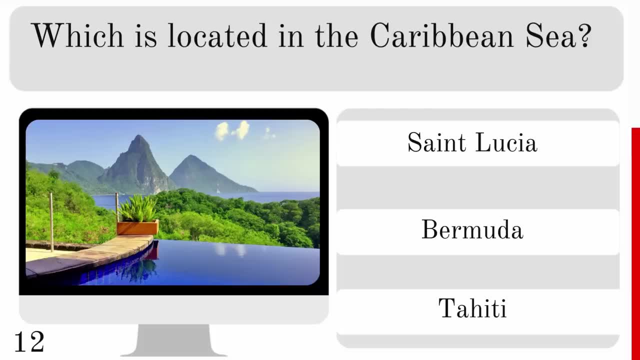 And they are on the border of Brazil and Argentina. Which is located in the Caribbean Sea? Santa Lucia, Bermuda or Tahiti, And the only one there that's in the Caribbean is St Lucia, Which ocean has the warmest surface temperature of the world's oceans. 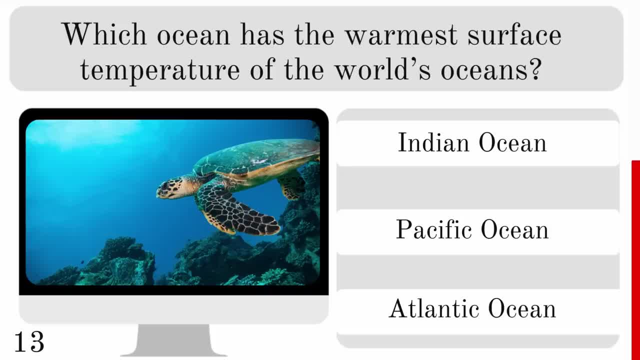 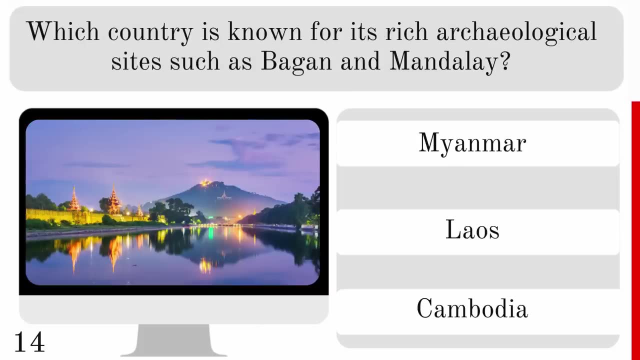 The Indian, Pacific or Atlantic, And the warmest is the Indian Ocean. Which country is known for its rich archaeological sites, such as Bagan and Mandalay? Myanmar, Laos or Cambodia? And the correct answer is Myanmar. What is the highest mountain in Africa? 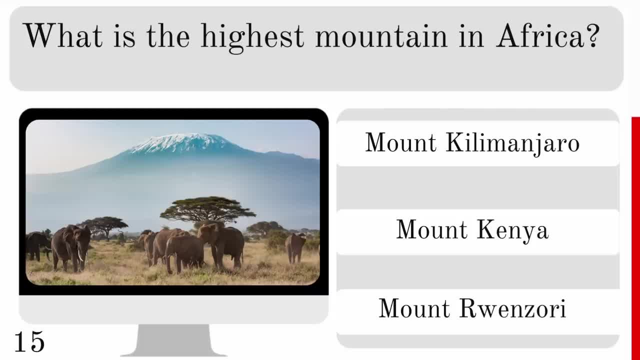 Is it Mount Kilimanjaro, Kenya or Renzori? And the highest is Mount Kilimanjaro. Which country is known for its rich archaeological sites, such as Bagan and Mandalay? Which US city is known as the Windy City? 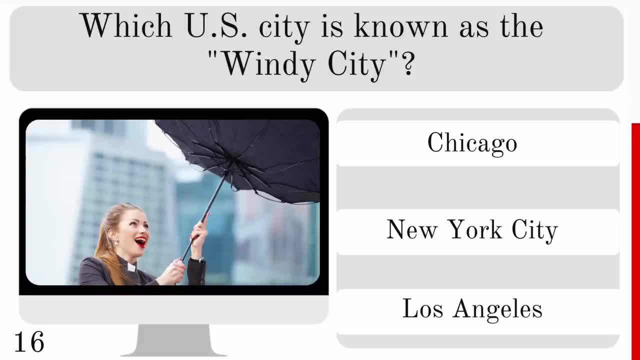 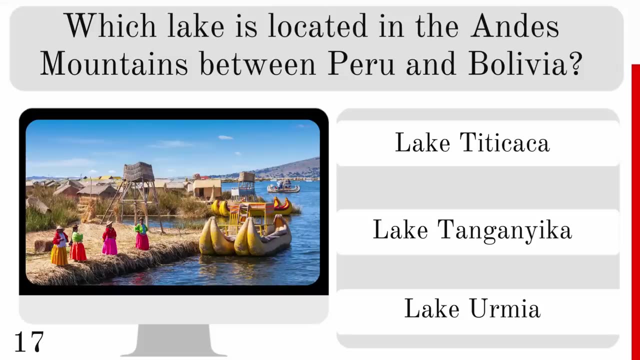 Is it Chicago, New York City or Los Angeles? And the Windy City is Chicago. Which lake is located in the Andes Mountains between Peru and Bolivia? Is it Lake Titicaca, Tanganyika or Urmia? And the correct answer is Lake Titicaca. 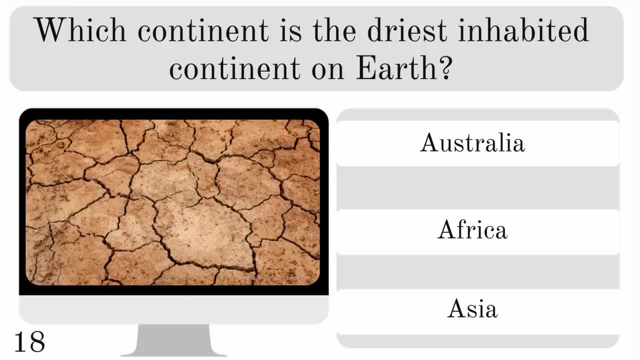 And the correct answer. Which continent is the driest inhabited continent on Earth? Australia, Africa or Asia? And the answer is Australia. Which country is known as the Rainbow Nation? South Africa, Peru or Canada? And the correct answer is Canada. 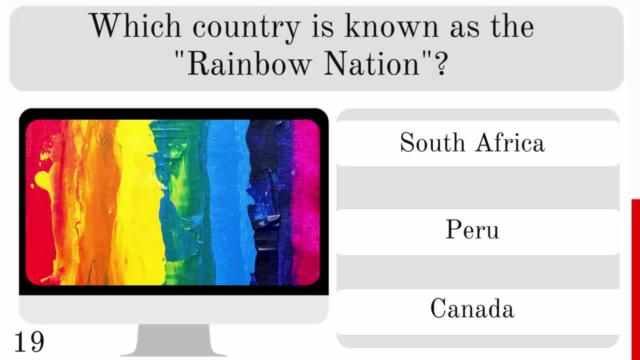 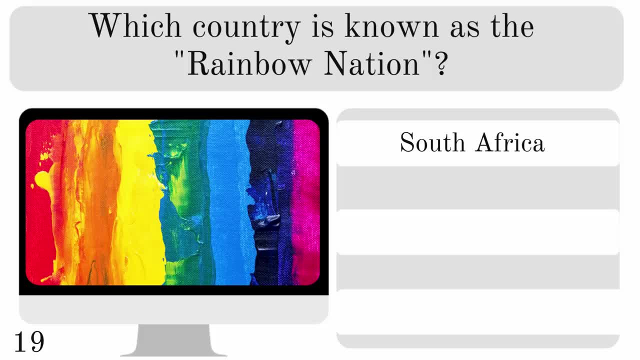 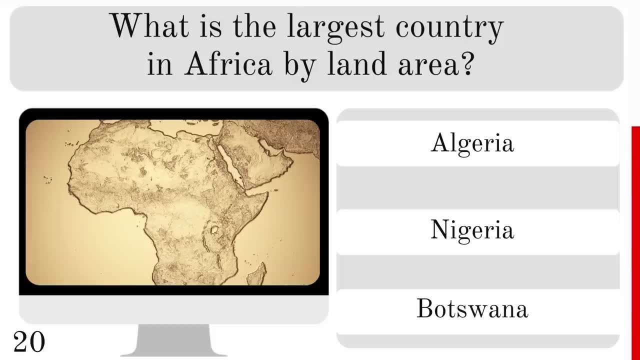 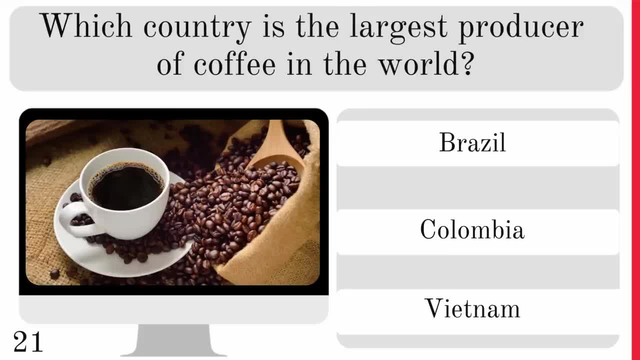 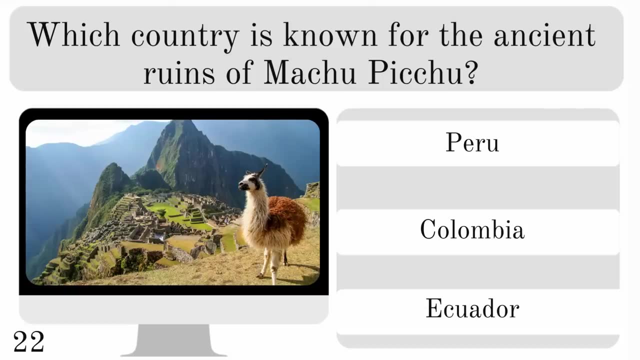 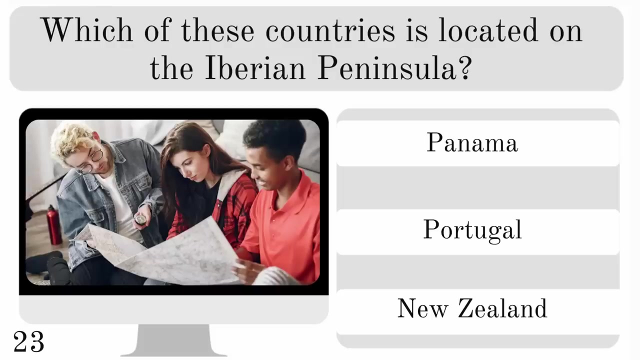 Which country is the largest producer of coffee in the world? Is it Brazil, Colombia or Vietnam? Is it Colombia, Facebook, France or Mexico? The answer is Brazil. Which country is known for the ancient ruins of Machu Picchu? Peru, Colombia or Ecuador? 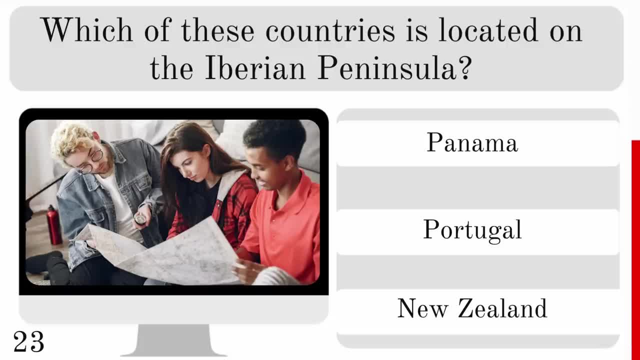 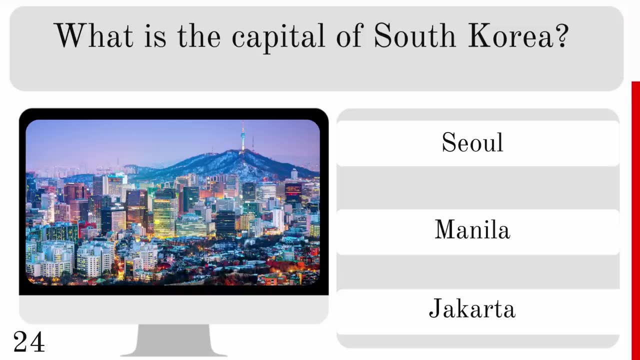 And they are found in Peru. Which of these countries is located on the Iberian Peninsula? Panama, Portugal or New Zealand? Panama, Portugal or New Zealand? The correct answer is Portugal. What is the capital of South Korea? Is it Seoul, Manila or Jakarta? 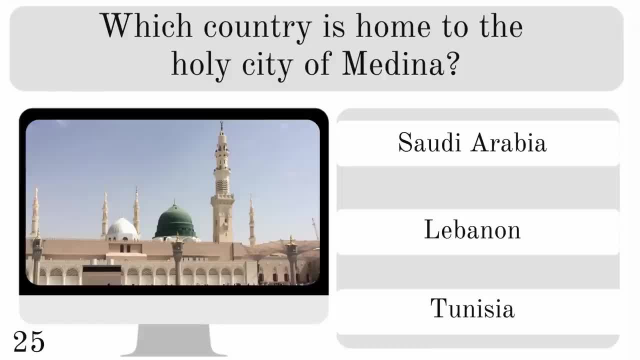 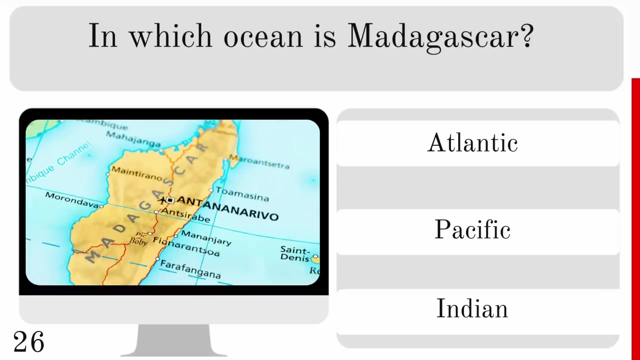 And it is Seoul. Which country is home to the holy city of Medina? Saudi Arabia, Lebanon or Tunisia? That is in Saudi Arabia. In which ocean is Madagascar? The Atlantic, Pacific or Indian? And it's in the Indian Ocean. What is the largest country in the Caribbean? 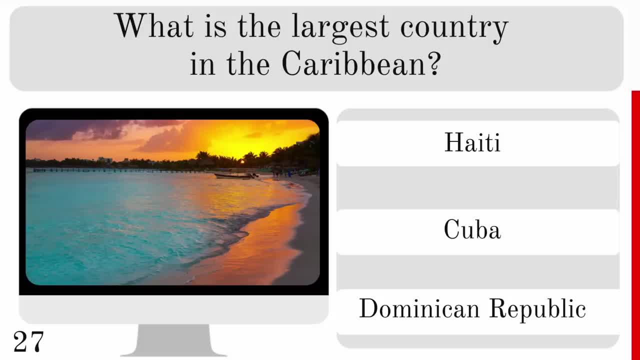 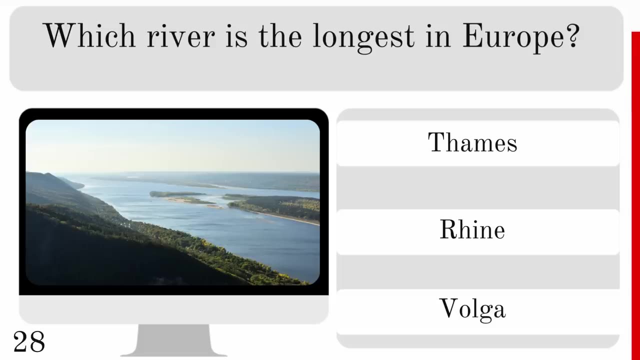 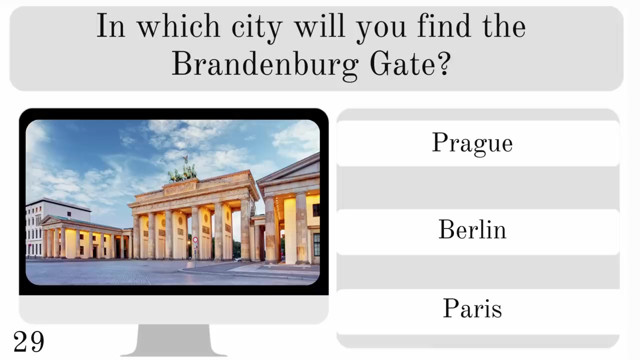 Is it Haiti, Cuba or the Dominican Republic? And the largest is Cuba. Which river is the longest in Europe- The Thames, Rhine or Volga? And the longest there is the Volga. In which city will you find the Brandenburg Gate? Prague, Berlin or Paris? And it's in Berlin. In which country is Lake Como located? Italy, Spain or Switzerland? The answer is Italy. What is the capital of Argentina? Is it Buenos Aires, Santiago or Lima? And the answer is Buenos Aires. 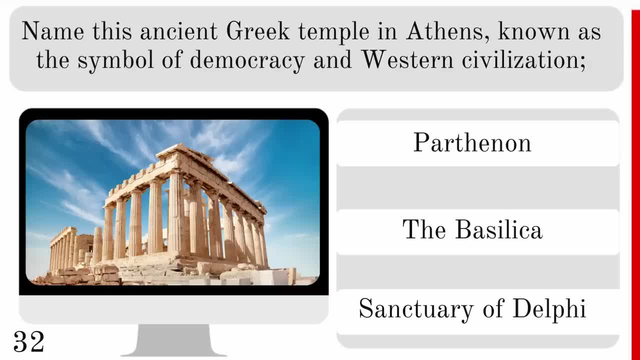 Name this Greek temple in Athens, known as the symbol of democracy and western civilization? Is it the Parthenon, the Basilica or the Sanctuary of Delphi? And the correct answer is the Parthenon. And the correct answer is the Parthenon. 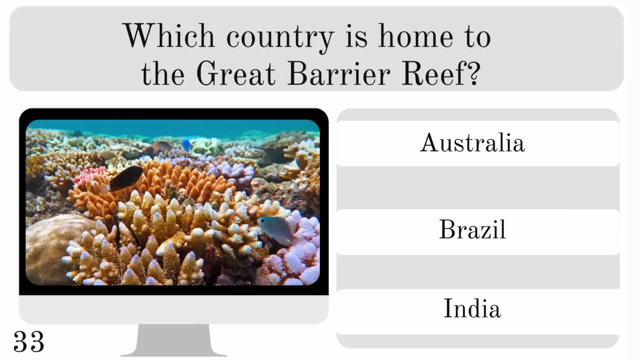 And the correct answer is the Parthenon. The Parthenon: Which country is home to the Great Barrier Reef? Is it Australia, Brazil or India? Is it Australia, Brazil or India? Is it Australia, Brazil or India? And the correct answer is Australia. 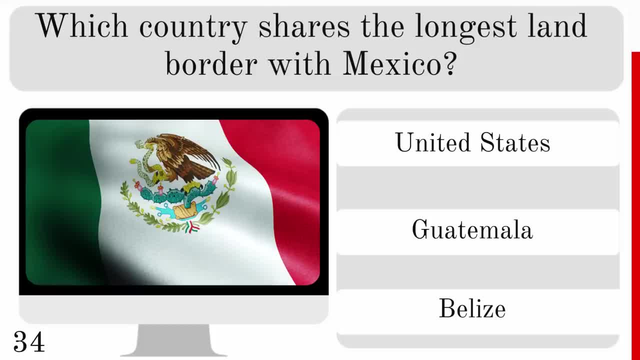 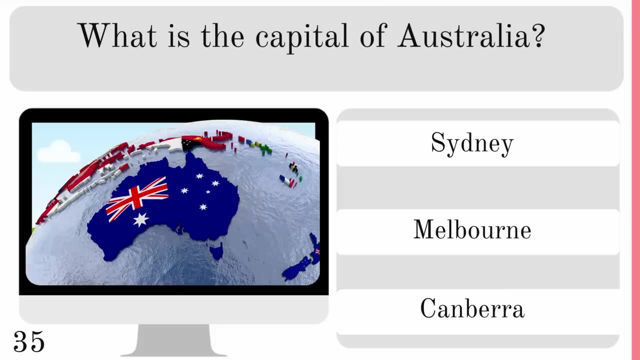 Which country shares the longest land border with Mexico? the United States, Guatemala or Belize? The United States, Guatemala or Belize? The United States, Guatemala or Belize? The United States, Venezuela or Belize? The right answer is France, the United States. What is the capital of Australia? Is it Sydney, Melbourne or Canberra? 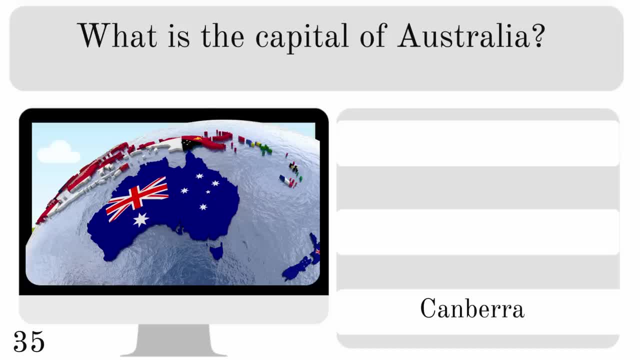 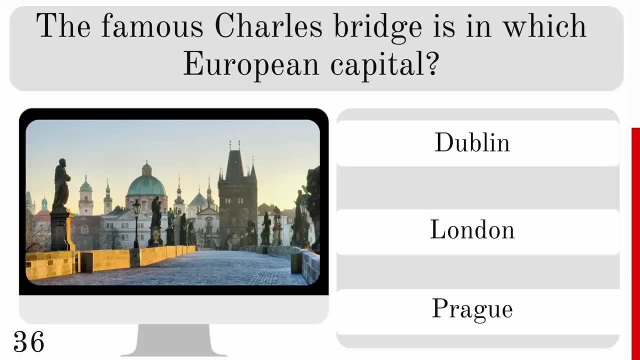 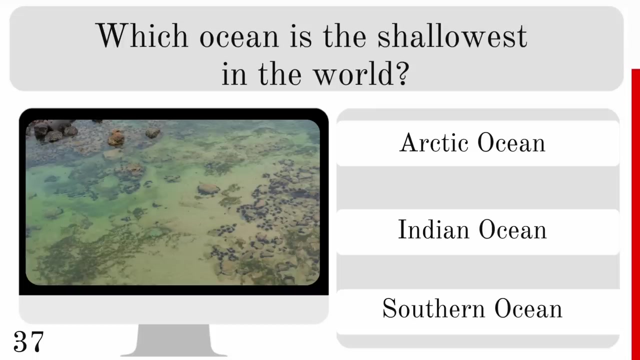 And the answer is Canberra. The famous Charles Bridge is. in which European capital? Is it Dublin, London or Prague? And that is in Prague. Which ocean is the shallowest in the world? The Arctic, Indian or Southern? And the shallowest is the Arctic Ocean. Which. 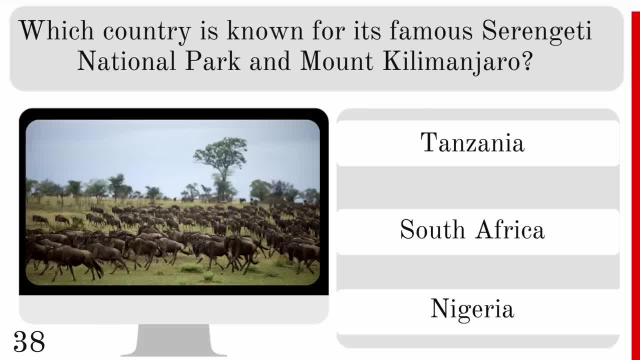 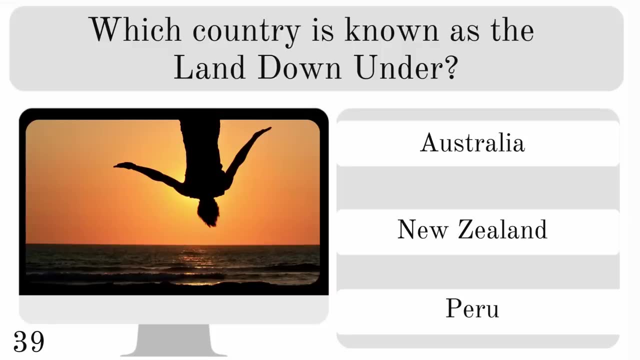 country is known for its famous Serengeti National Park and Mount Kilimanjaro? Tanzania, South Africa or Nigeria? The correct answer: Tanzania. Which country is known as the Land Down Under? Australia, New Zealand or Peru? And the correct. 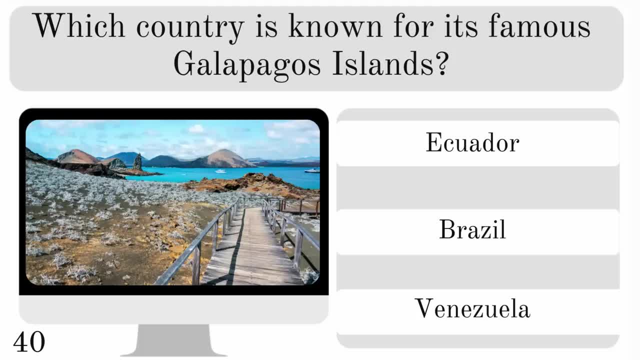 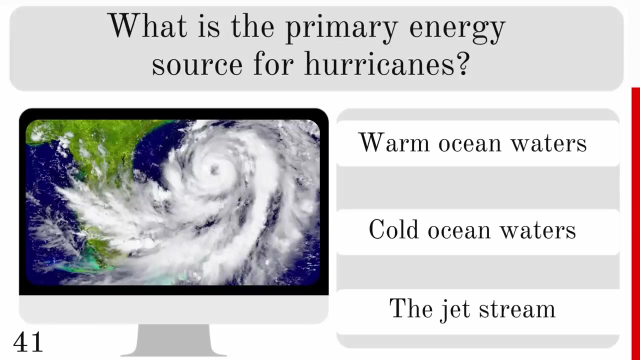 answer: Australia. Which country is known for its famous Galapagos Islands? Ecuador, Brazil or Venezuela, And they belong to Ecuador. What is the primary energy source for hurricanes? Is it warm ocean waters, cold ocean waters or the jet stream? 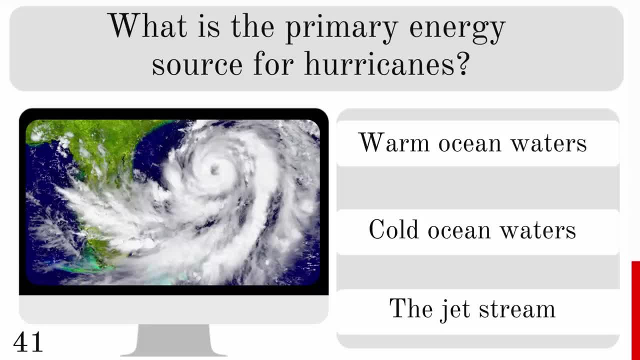 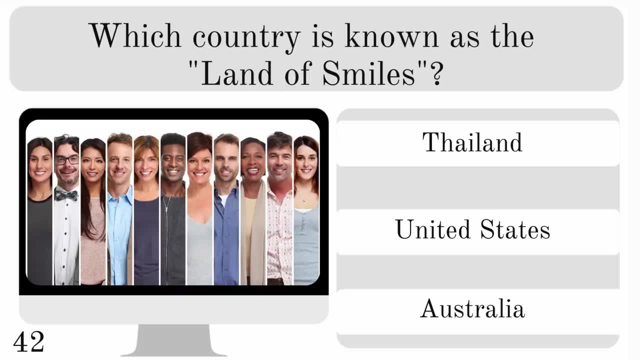 The correct answer is the warm ocean waters, And the answer is warm ocean waters. Which ocean is known for its famous Galapagos Islands, Ecuador, Brazil or Venezuela? The correct answer: Which country is known as the land of smiles? Thailand, the United States or Australia? 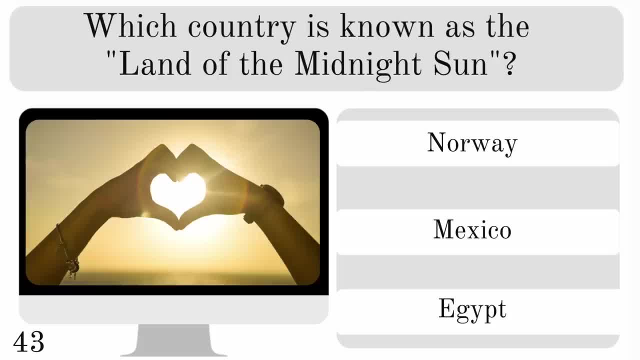 And the answer there is Thailand. And which country is known as the land of the midnight sun? Norway, Mexico or Egypt? The correct answer is Norway. Which country is known for its vast pampas stakes and the love for tango Argentina? 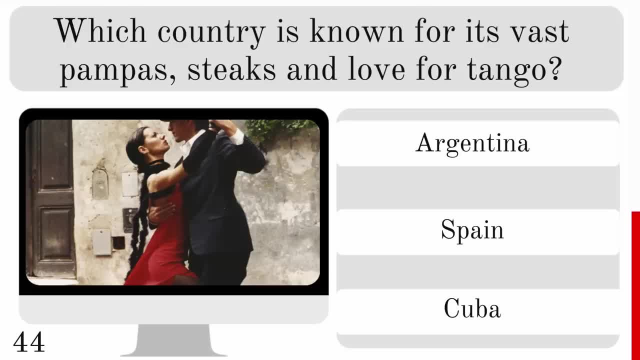 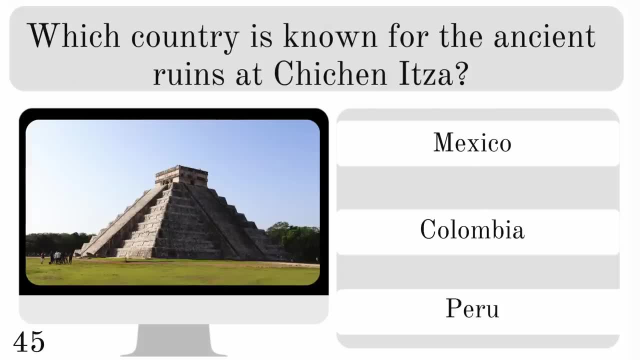 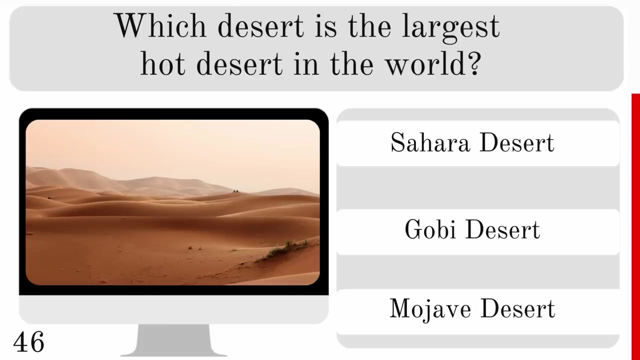 Spain or Cuba. The correct one there is Argentina. Which country is known for the ancient ruins at Chichen Itza? Mexico, Colombia or Peru? And that's located in Mexico. Which desert is the largest hot desert in the world? Is it the Sahara, Gobi or Mojave? 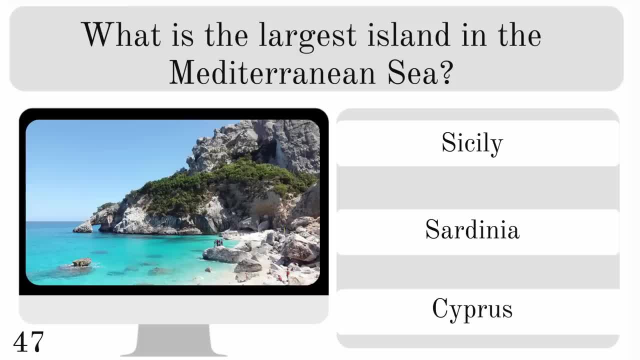 And the correct answer: the Sahara Desert. What is the largest island in the Mediterranean Sea? Is it Sicily, Sardinia or the Caribbean? The correct answer is the Sahara Desert. What is the largest island in the Mediterranean Sea? Is it the Sahara, Gobi or Mojave? 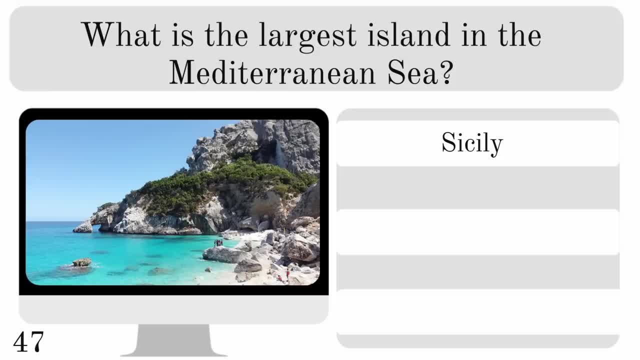 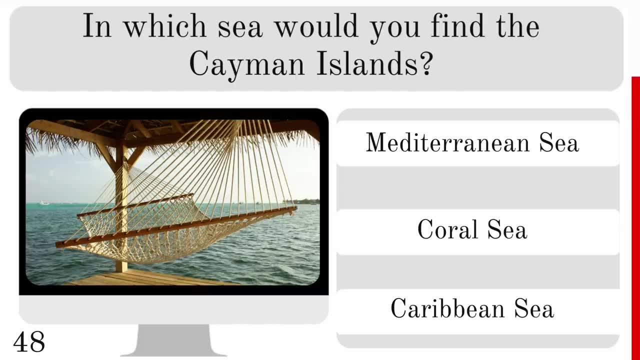 The correct answer is the Sahara Desert. In which sea would you find the Cayman Islands? Are they in the Mediterranean, Coral or Caribbean Sea? And they are located in the Caribbean. Which country does this flag belong to? France, Germany or Spain? 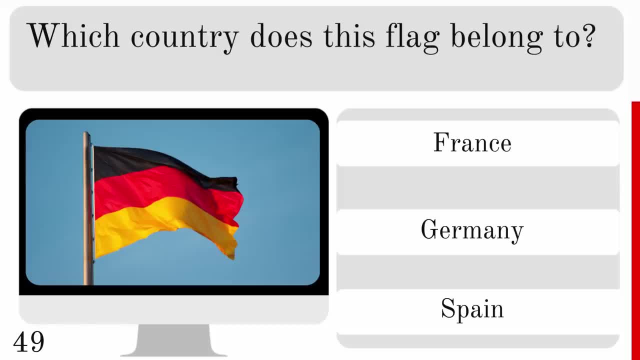 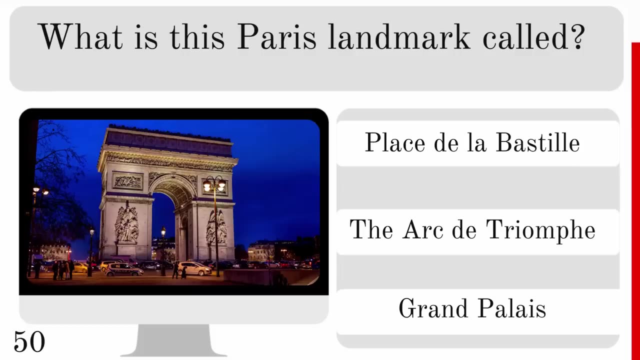 The correct answer is the Caribbean, France, Germany or Spain. And that is the flag of Germany. What is this Paris landmark called? Is it the Place de la Bastille, the Arc de Triomphe or the Grand Palais? And it is the Arc de Triomphe. 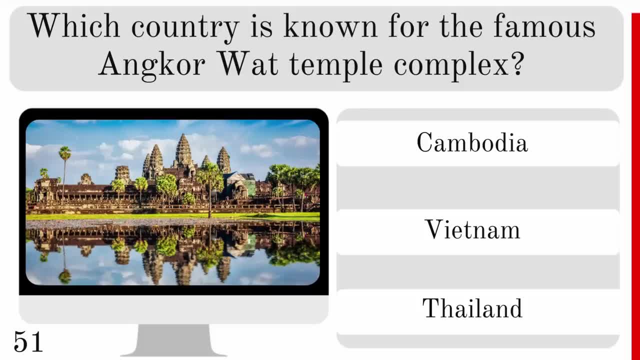 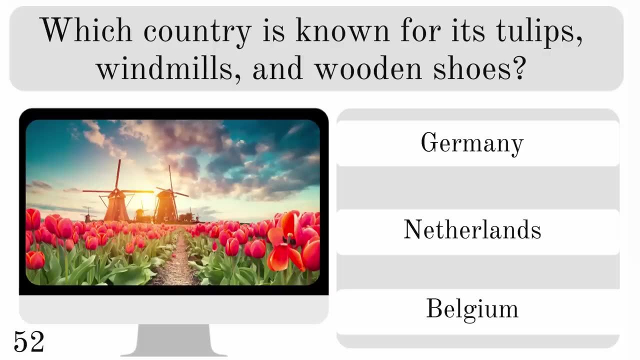 Which country is known for the famous Angkor Wat temple complex? Cambodia, Vietnam or Thailand, And that is in Cambodia. Which country is known for its tulips, windmills and wooden shoes? Germany, Netherlands or Belgium, And the correct answer: the Netherlands. 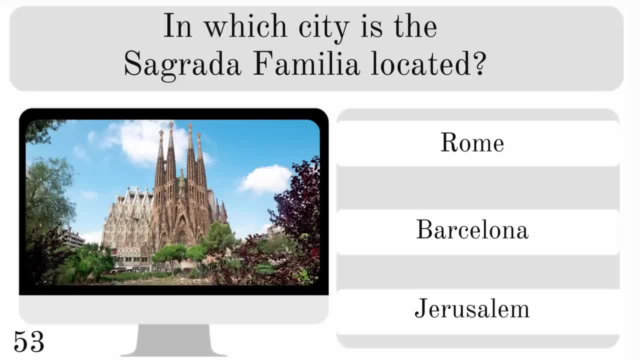 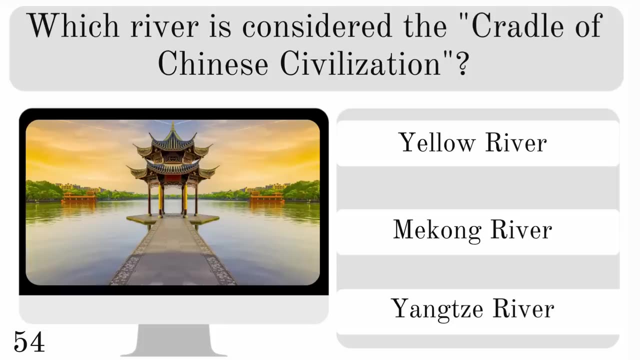 Okay. In which city is the Sagrada Familia located? Is it in Rome, Barcelona or Jerusalem? And it is in Barcelona. Which river is considered the cradle of Chinese civilization? The Yellow Mekong or Yangtze? 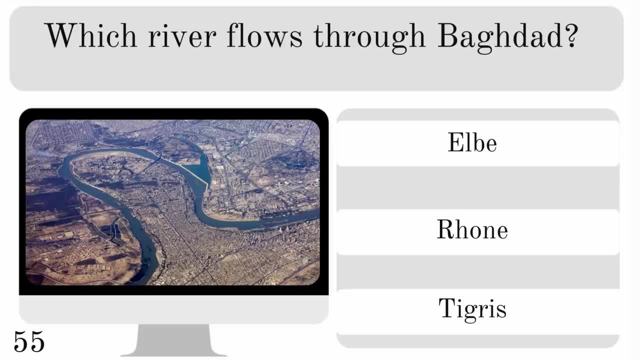 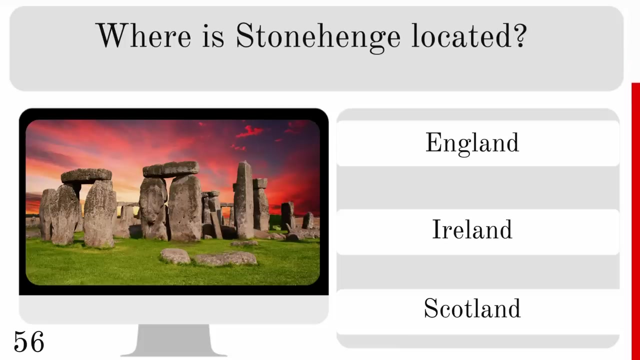 And the answer: the Yellow River. Which river flows through Baghdad, the Elbe, Rhone or Tigris? And the answer: the Tigris. Where is Stonehenge located? Is it in England, Ireland or Scotland? And it is in Scotland. 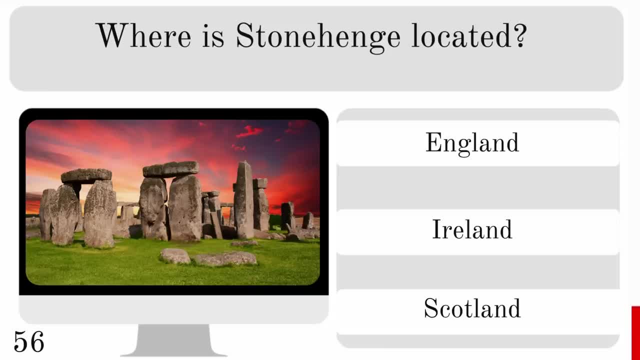 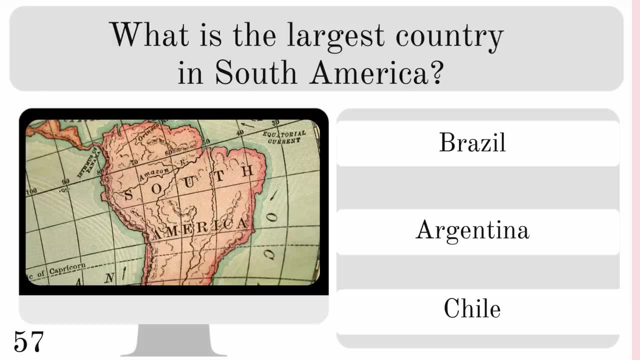 And it is in England, Ireland or Scotland, And it is in England. Ireland or Scotland, And it is in Scotland, And it is in Scotland And it's in England. What is the largest country in South America? Is it Brazil, Argentina or Chile? 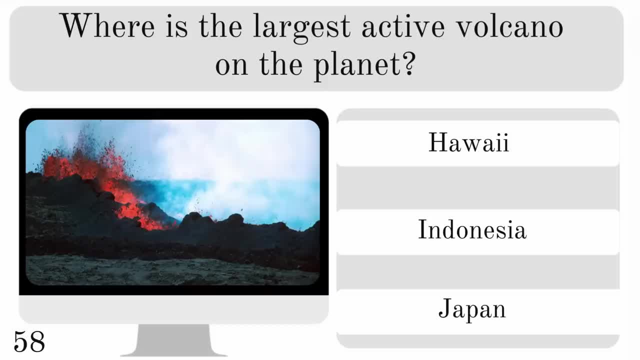 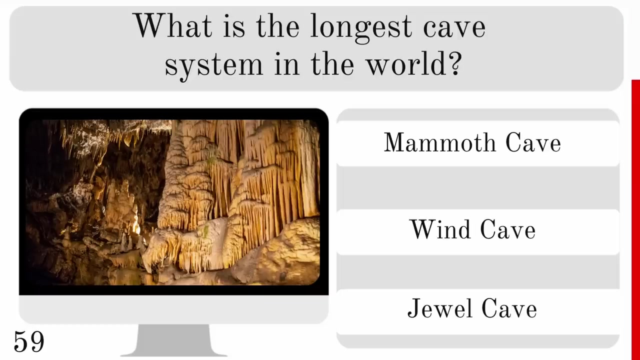 And the answer is Brazil. Where is the largest active volcano on the planet? Is it in Hawaii, Indonesia or Japan? And it's in Hawaii. What is the longest cave system in the world? Is it Mammoth Wind or Jewel Cave? 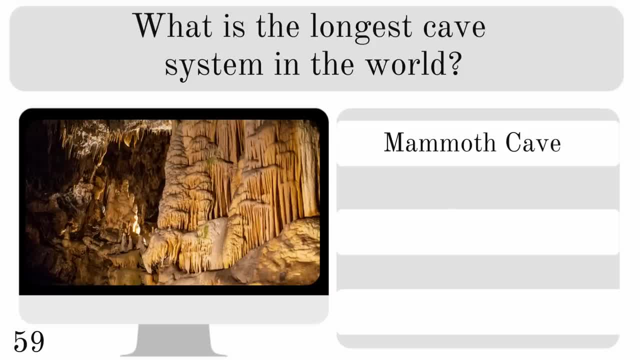 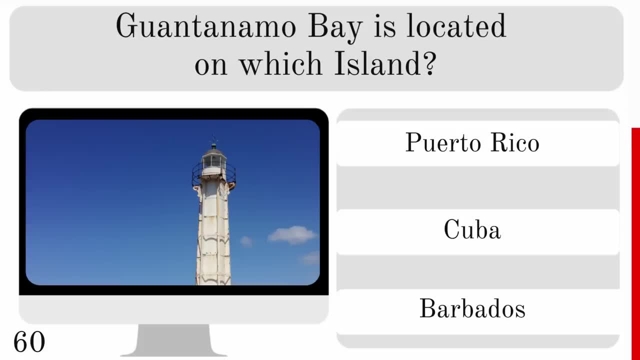 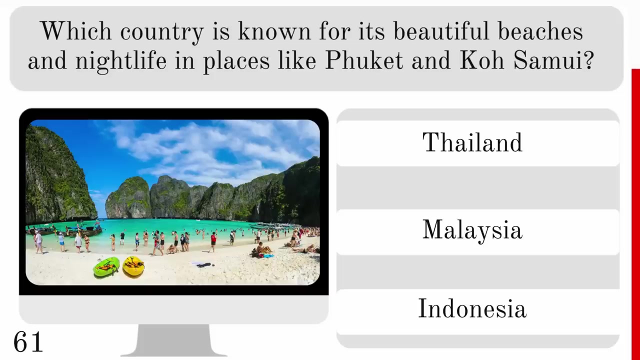 And the correct answer. Mammoth Cave, Guantanamo Bay, is located on which island? Puerto Rico, Cuba or Barbados? And it's on Cuba Which country is known for its beautiful beaches and nightlife in places like Phuket and Koh Samui. 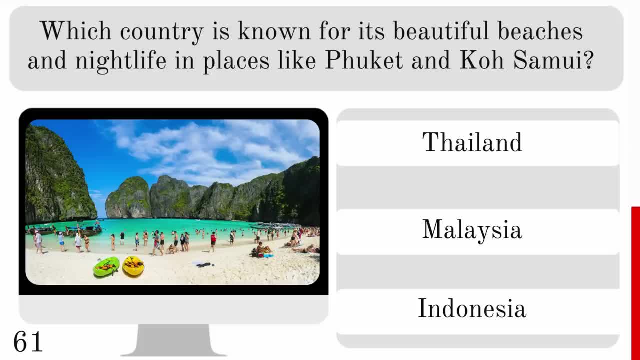 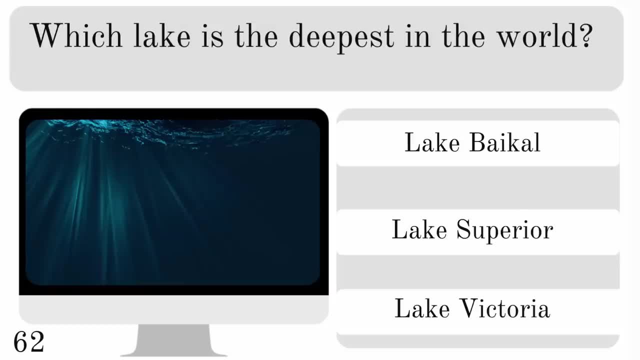 Thailand, Malaysia or Indonesia, And the correct answer is Thailand. Which lake is the deepest? The deepest lake in the world? Lake Baikal, Superior or Victoria, And the correct answer: Lake Baikal. Which mountain range is known for its iconic peaks such as the Matterhorn and Eiger? 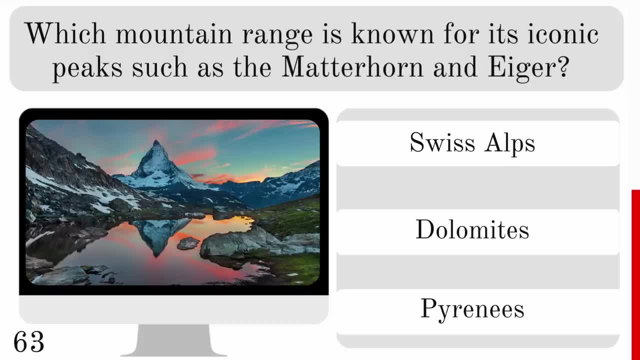 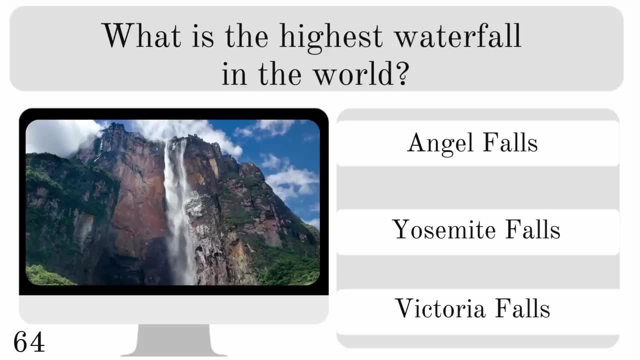 Is it the Swiss Alps, Dolomites or Pyrenees? And the correct answer the Swiss Alps, And the correct answer the Swiss Alps. What is the highest waterfall in the world? Angelfalls, Yosemite Falls or Victoria Falls? 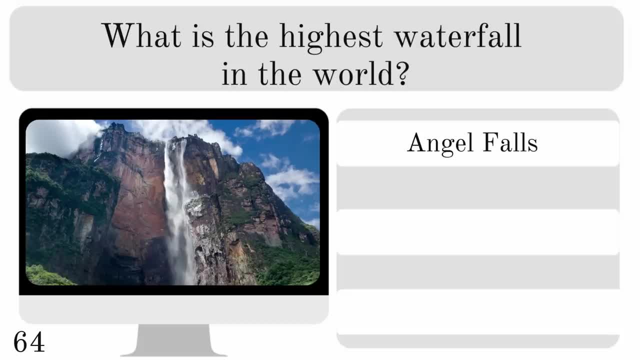 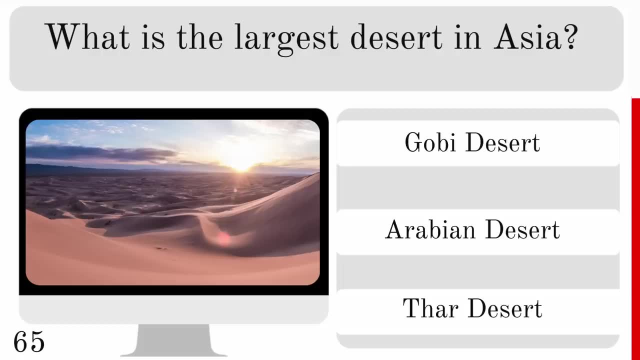 And the correct answer is Angelfalls. What is the largest desert in Asia? Is it the Gobi, Arabian or Thar? And the largest in Asia is the Arabian Sea. Is it the Gobi, Arabian or Thar? And the largest in Asia is the Arabian Sea. 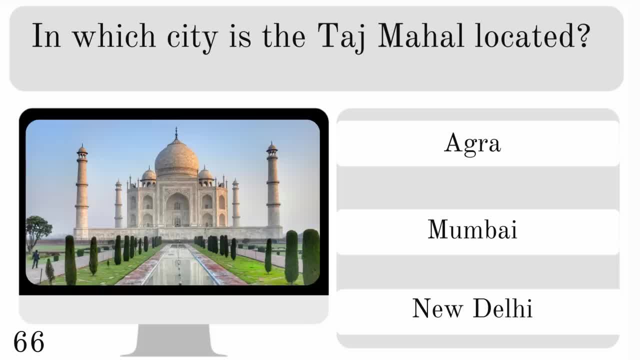 What is the highest mountain in the world? Arabian desert? In which city is the Taj Mahal located? Is it in Agra, Mumbai or New Delhi? And that's found in Agra. Which country is known as the land of the rising sun? China, Japan or New Zealand? 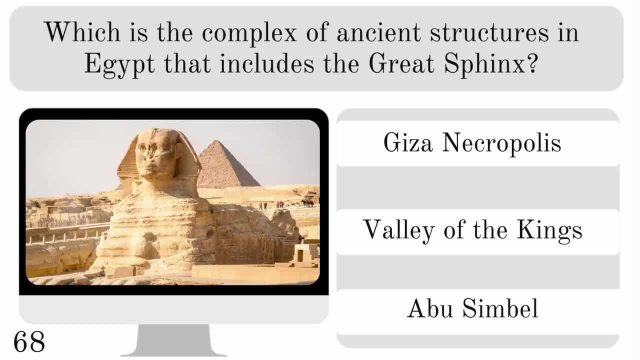 The answer there is Japan, Which is the complex of ancient structures in Egypt. that includes the Great Sphinx, The Giza Necropolis, the Valley of the Kings or Abu Simbul. And the correct answer there: the Giza Necropolis. What is the highest capital city in the world? Is it La Paz, Kathmandu or Bogota? 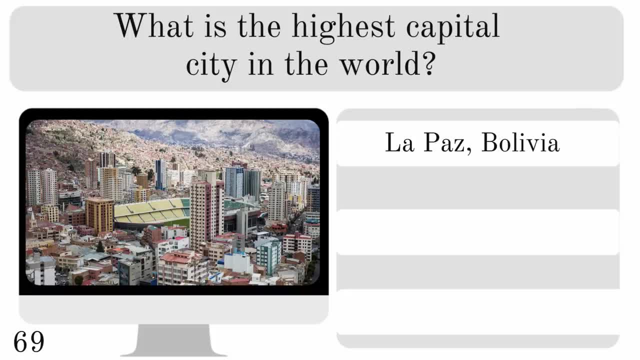 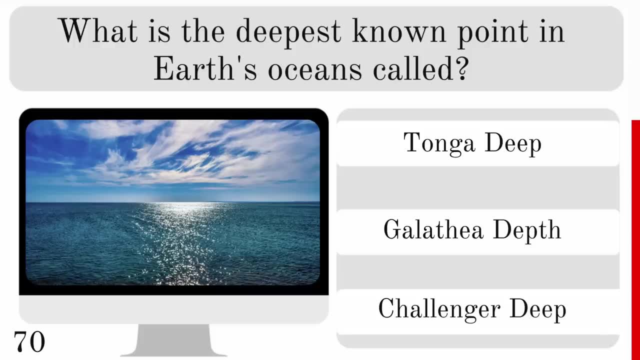 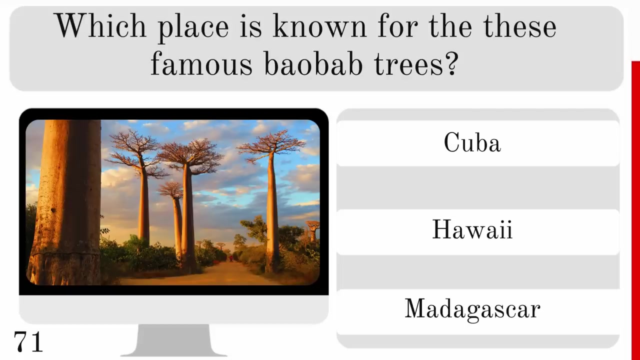 And the correct answer: La Paz, Bolivia. What is the deepest known point in the Earth's oceans called? Is it the Tonga, Galathea or Challenger Deep? And the correct answer: the Challenger Deep. Which place is known for these famous baobab trees? Is it Cuba, Hawaii or Madagascar? 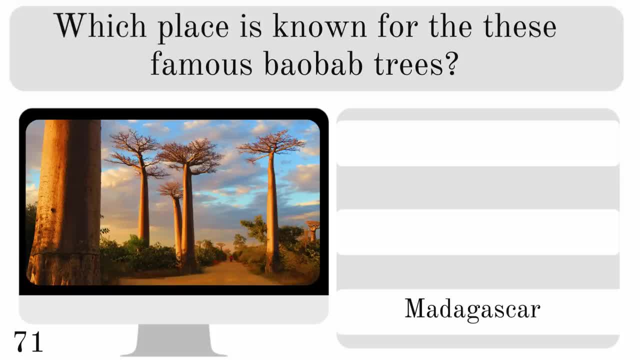 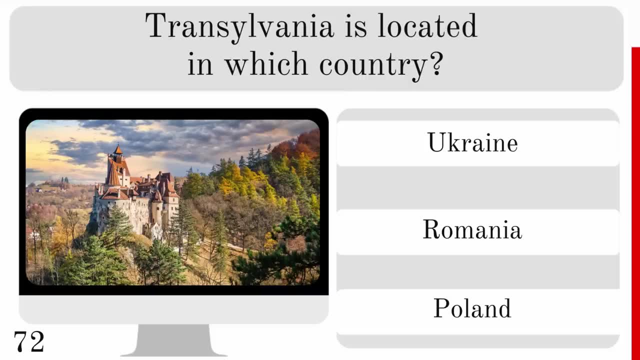 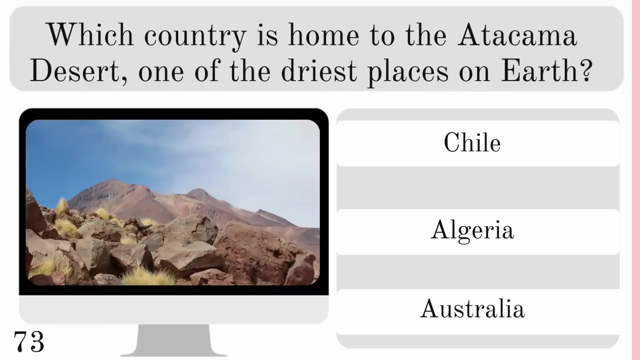 And they are found in Madagascar. Transylvania is located in which country? The Ukraine, Romania or Poland? And it's in Romania. Which country is home to the Atacama Desert, one of the driest places on Earth? Is it in Chile, Algeria or Australia? 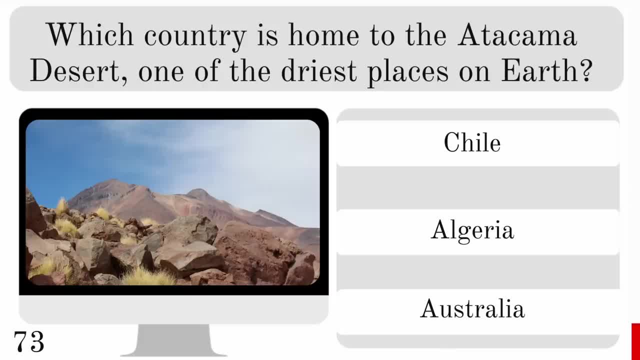 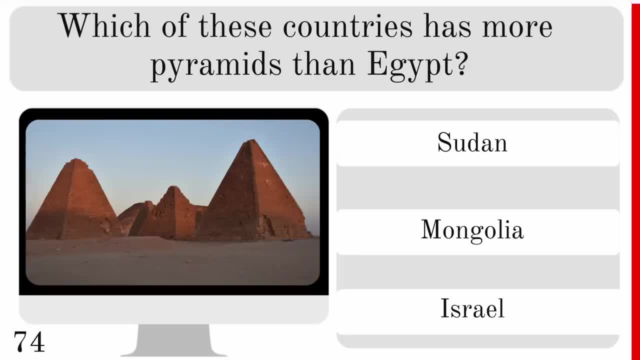 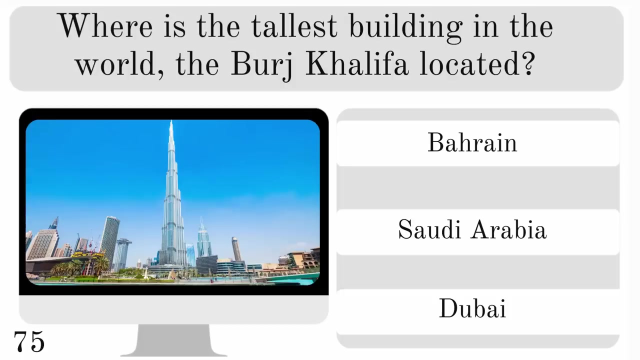 And it's found in Chile. Which of these countries has more pyramids than Egypt, Sudan, Mongolia or Israel? And the correct answer: Sudan. Where is the tallest building in the world, the Burj Khalifa, located? Is it in Bahrain, Saudi Arabia or Dubai? 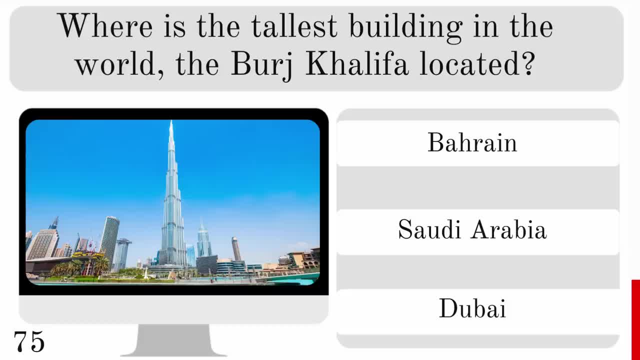 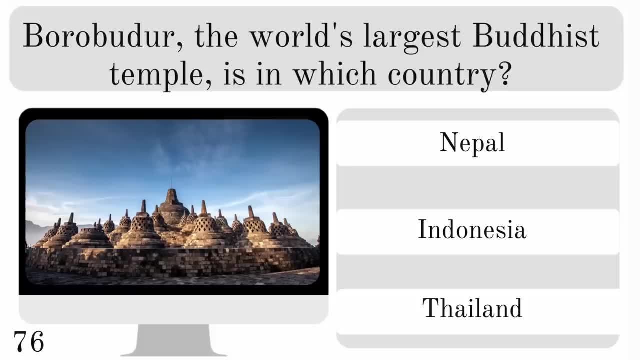 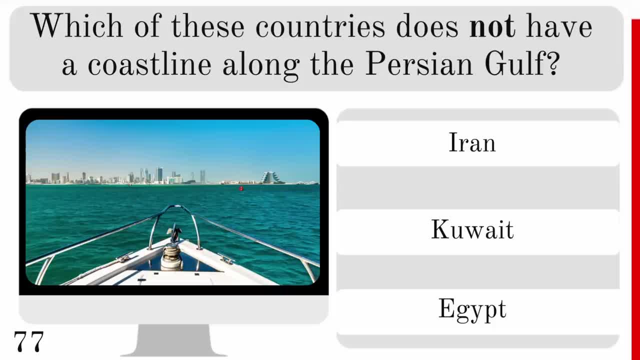 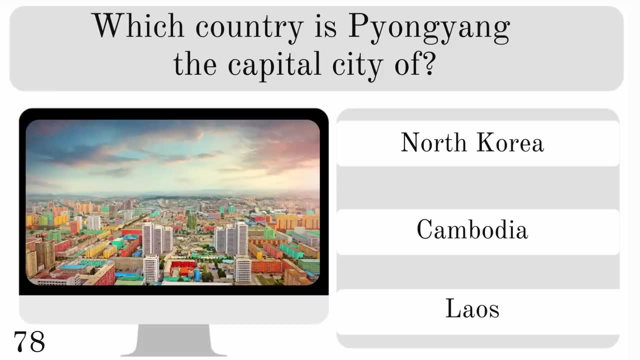 Which of these countries does not have a coastline along the Persian Gulf? Iran, Kuwait or Egypt? The North Korean capital, Mexico or the West dead Delhi? And it's in? And the answer there is Egypt. Which country is Pyongyang, the capital city of North Korea? Cambodia or Laos? 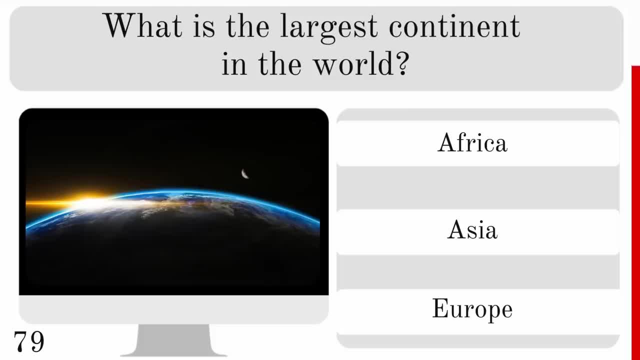 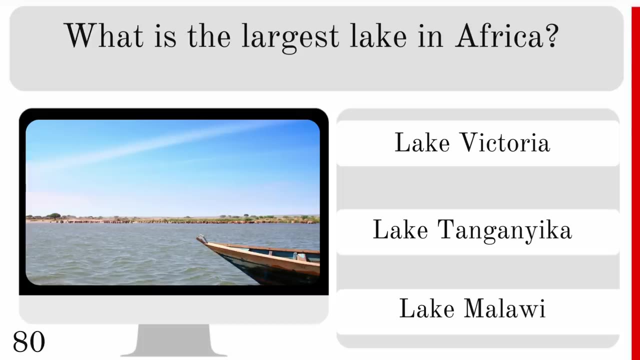 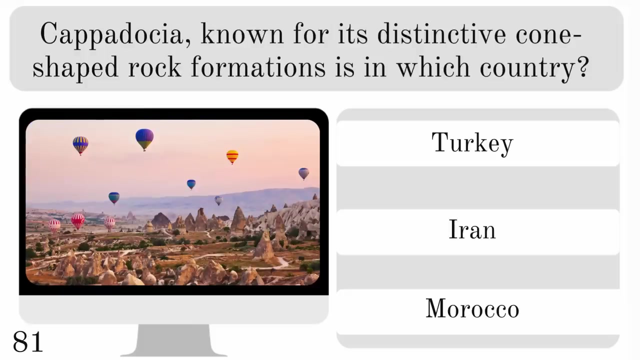 And it's the capital of North Korea, And the largest is Asia. What is the largest lake in Africa? Is it Lake Victoria, Tanganyika or Malawi? And the largest is Lake Victoria, Cappadocia, known for its distinctive cone-shaped rock formations, is in which country? 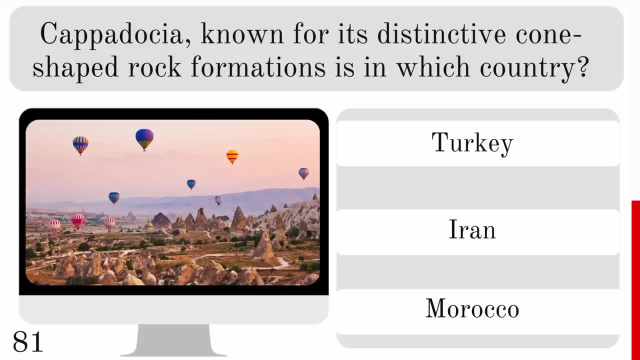 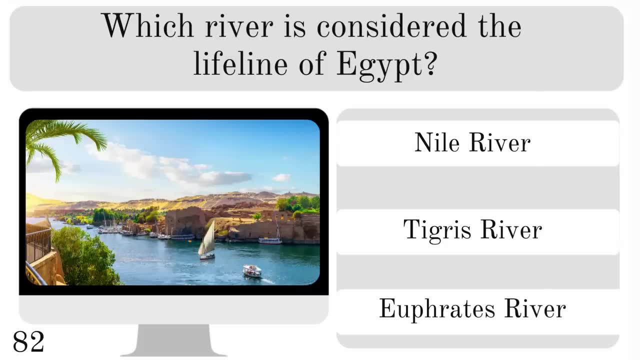 Turkey, Iran or Morocco, And it's found in Turkey. Which river is considered the lifeline of Egypt? The Nile, Tigris or Euphrates? And the correct answer: the Nile. Which country is the smallest in terms of land area? 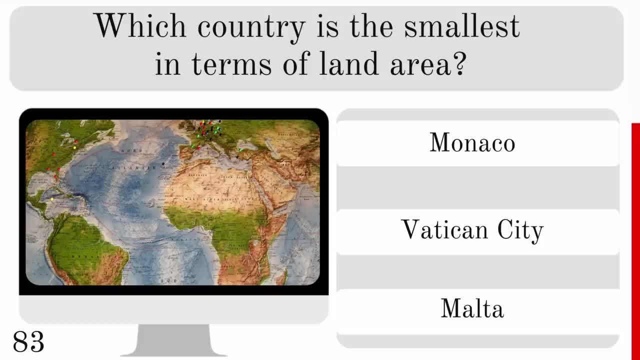 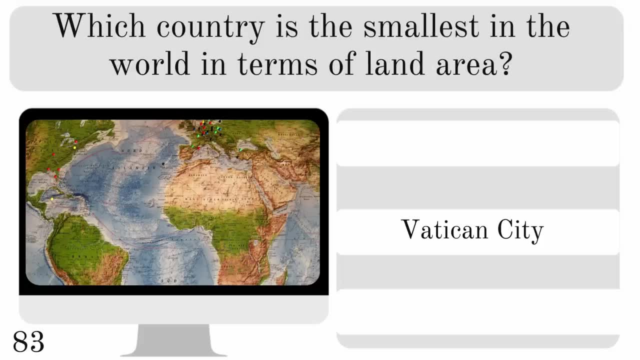 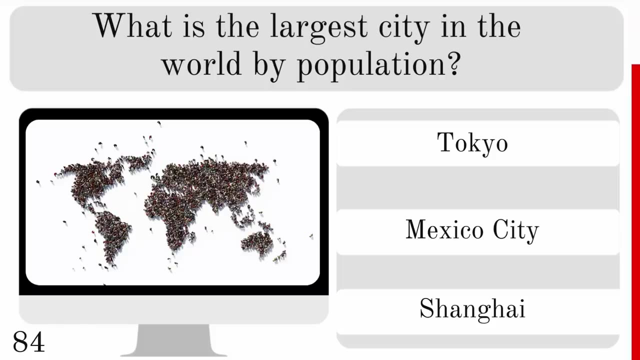 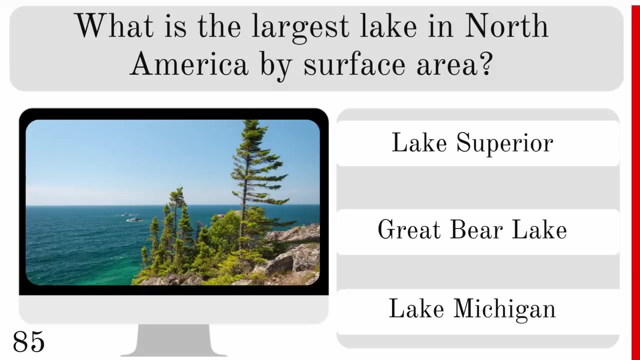 Monaco, Vatican City or Malta, And the smallest is Vatican City. What is the largest city in the world by population- Tokyo, Mexico City or Shanghai? And the answer there is Tokyo. What is the largest lake in North America by surface area? 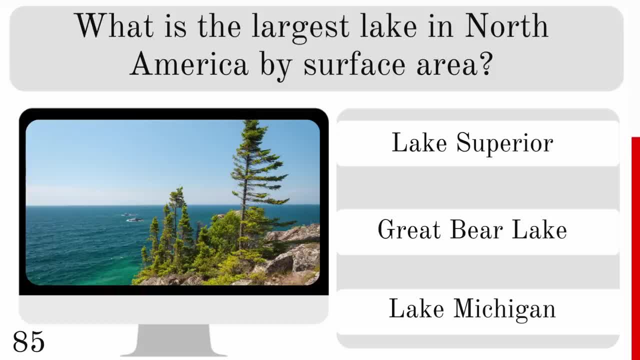 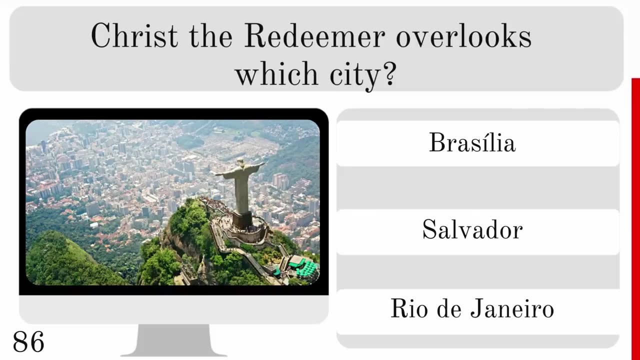 Is it Lake Superior, Great Bear Lake or Lake Michigan? And the answer is Lake Superior. Christ the Redeemer overlooks which city: Brasilia, Salvador or Rio de Janeiro? And the correct answer is Rio de Janeiro. And the correct answer is Rio de Janeiro. 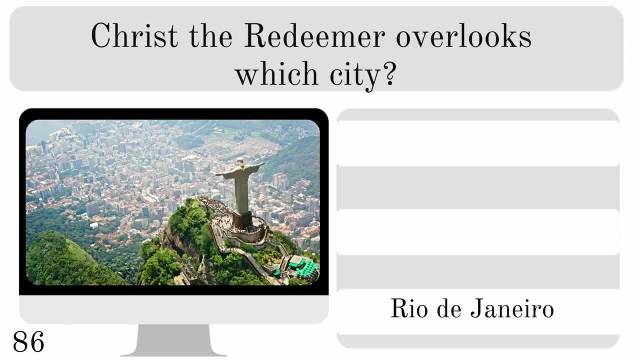 And the correct answer is Rio de Janeiro. Which country is known for its delicious chocolates, waffles and fries? Belgium, the United Kingdom or Austria? The answer there is Belgium. Which country is known for its delicious chocolates, waffles and fries? 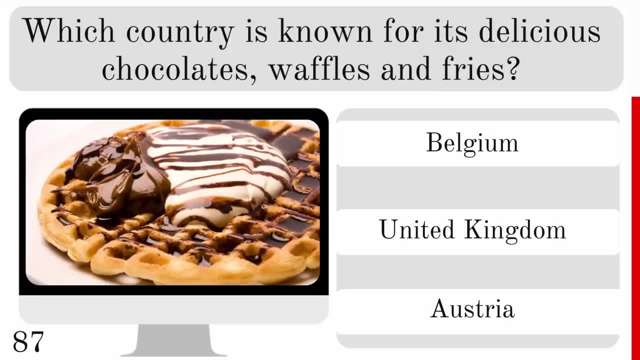 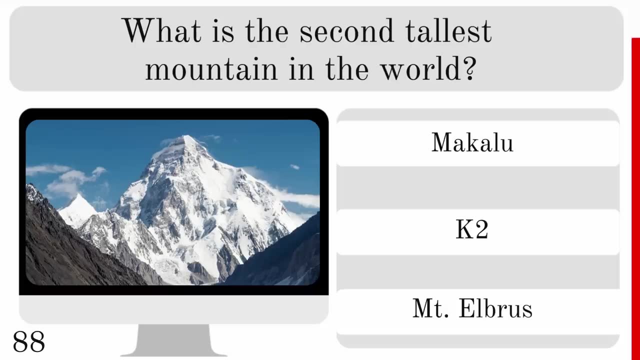 Belgium, the United Kingdom or Austria? The answer there is Belgium. What is the second tallest mountain in the world? Makalu K2 or Mount Elbrus? Makalu K2 or Mount Elbrus? And the correct answer is K2.. 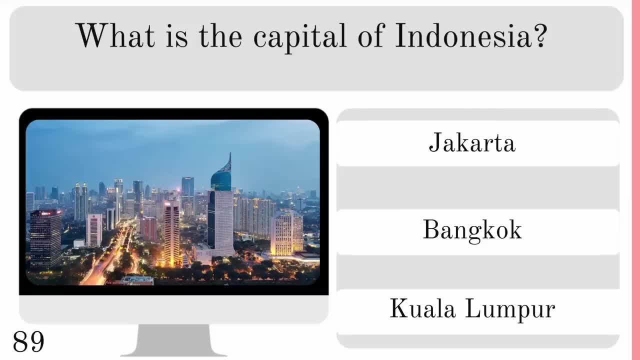 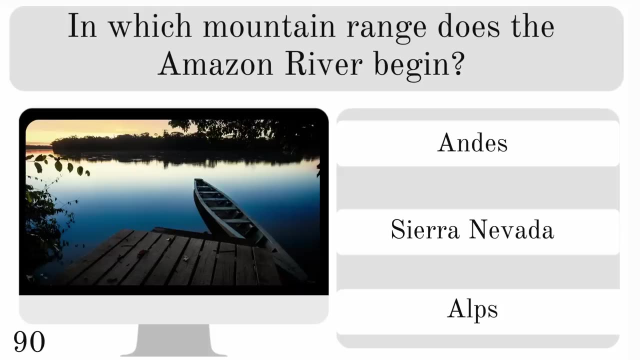 What is the capital of Indonesia? Is it Jakarta, Bangkok or Kuala Lumpur? And the correct answer: Jakarta. In which mountain range does the Amazon River begin? In the Andes, Sierra Nevada or Alps? And it begins in the Andes. 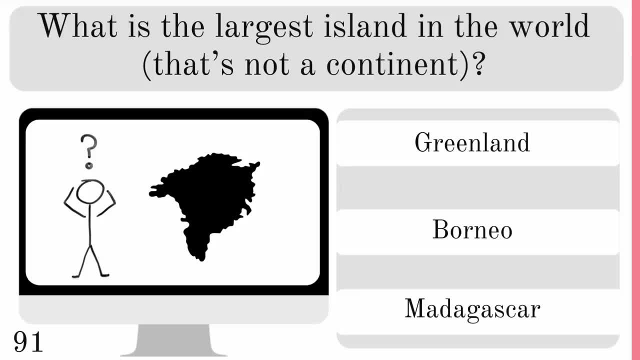 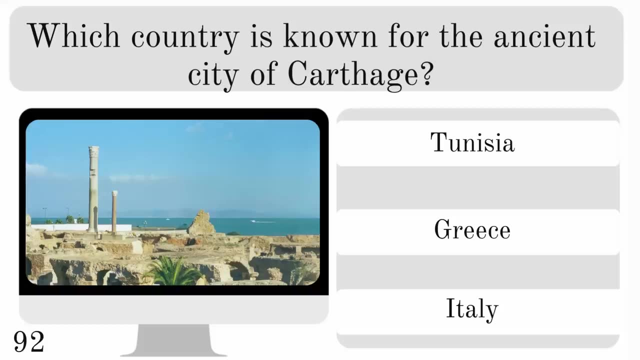 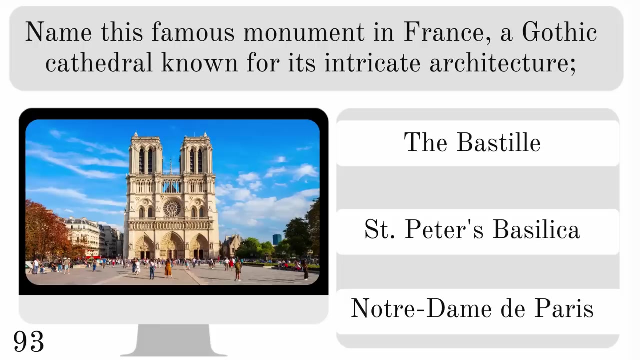 What is the largest island in the world? Greenland, Borneo or Madagascar? And the correct answer: Greenland. Which country is known for the ancient city of Carthage? Tunisia, Greece or Italy. The answer is: Tunisia. Name this famous monument in France, a Gothic cathedral known for its intricate architecture. 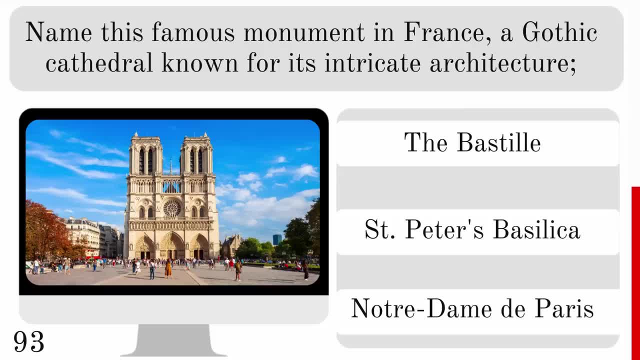 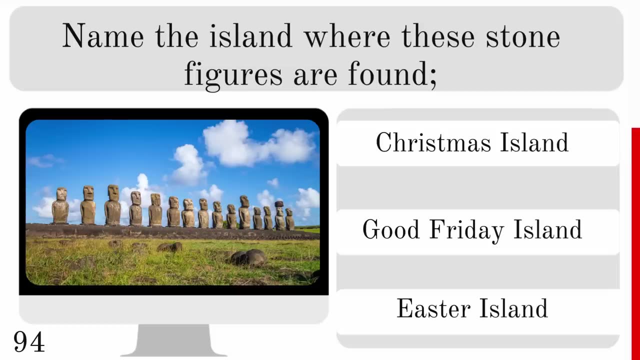 Is it the Bastille, St Peter's Basilica or Notre-Dame de Paris? And the answer is the Notre-Dame de Paris. Name the island where these stone figures are found. Is it Christmas, Good Friday or Easter Island? The answer is Christmas, Good Friday or Easter Island. 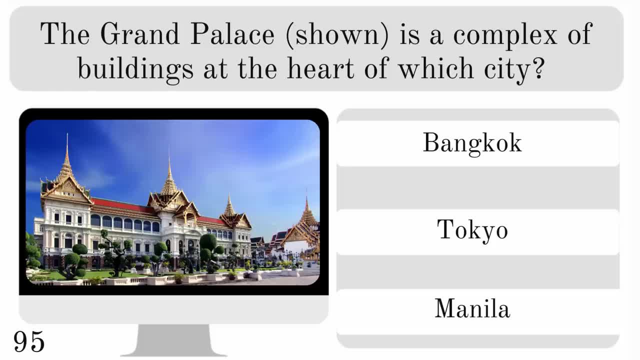 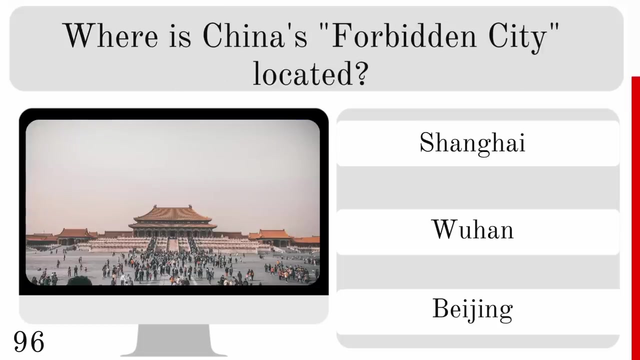 And they are found on Easter Island. The Grand Palace is a complex of buildings. in the heart of which city? Bangkok, Tokyo or Manila? And the correct answer is Bangkok. Where is China's Forbidden City located? Is it in Shanghai, Wuhan or Beijing? 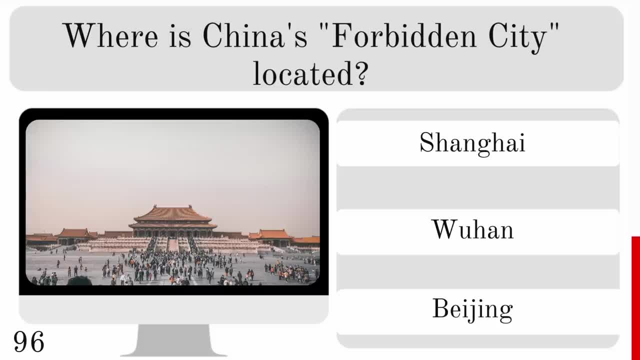 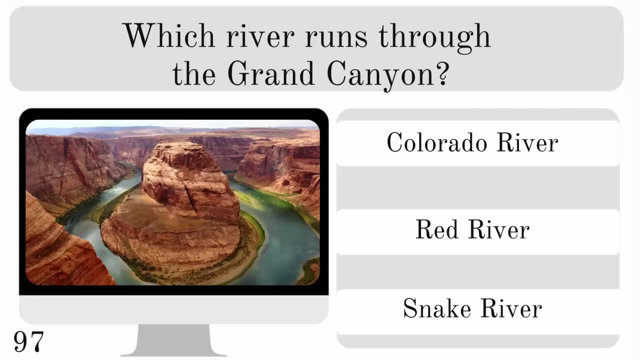 Yes, there is Shanghai, Wuhan or Beijing, But it is in Beijing, And it's in Beijing Which river runs through the Grand Canyon: The Colorado Red or Snake river, The Colorado Red or Snake river And the correct answer, the Colorado river.